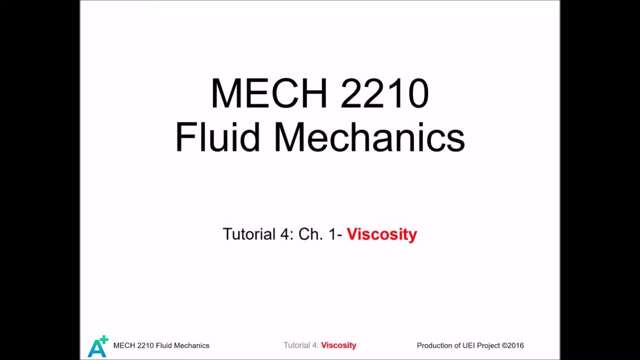 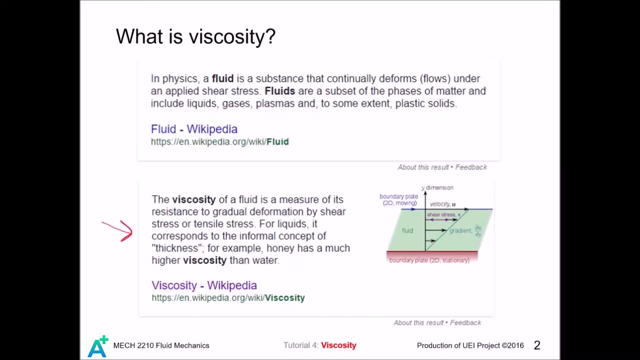 do spare some time to go through the examples and definitions in this video, since you are going to learn. viscous effect after the midterm. The definition of viscosity is given below in this paragraph It is defined as the resistance to gradual deformation, that is, flows by shear stress. In other words, that is the thickness of the fluid. 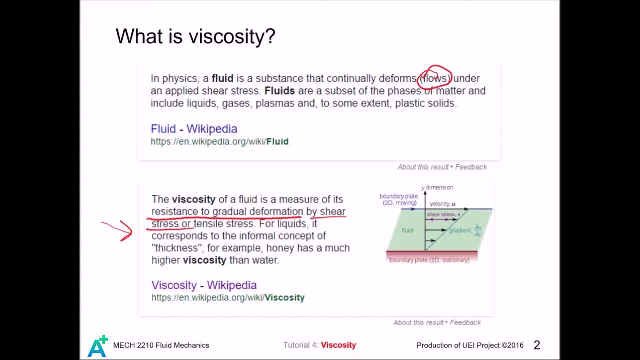 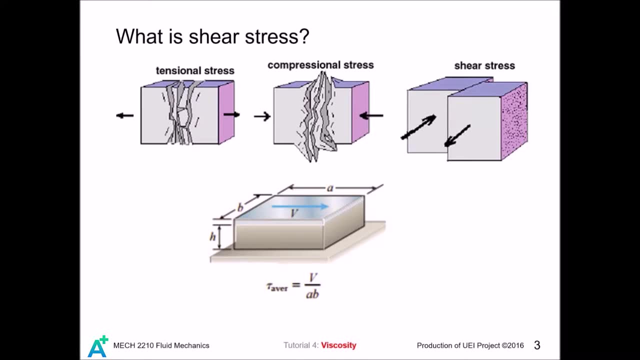 However, how can we measure such a thickness? What is shear stress? So let me help Lopez to teach some solid mechanics here. To represent internal forces, we usually draw pairs of opposite forces, Otherwise the material itself would accelerate. Tensile and compressional stress are rather intuitive. 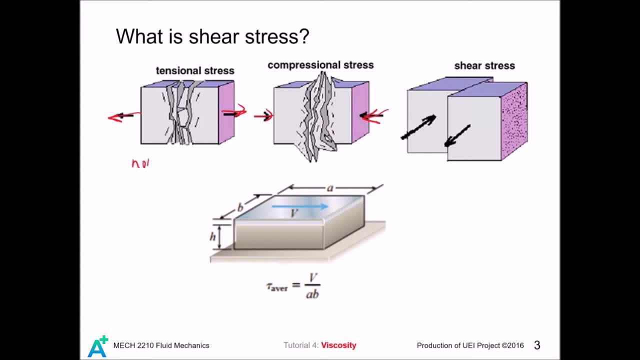 They act normal to the material cross-section, so they are often called normal stresses. But shearing stress is different. It acts coplanar to the material section. Shear is just another word for cut. Imagine that you have a pair of scissors here. 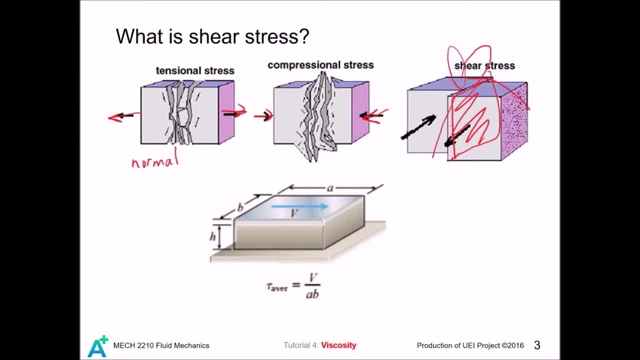 Then this will cut this piece of material into halves. Of course the direction of the cutting force is coplanar to the material section Down below here. if we have a pair of shearing forces, we must also take care of the reaction force. The shearing stress in a material is never uniform. 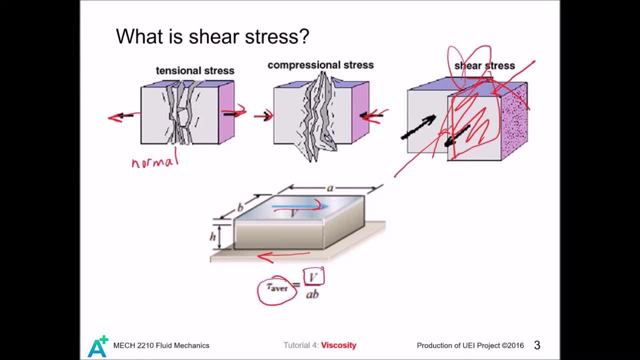 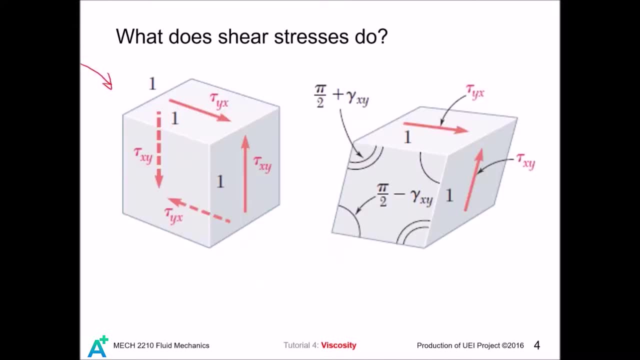 But the average shearing stress is the magnitude of one force divided by the area of the plane of action, that is Ab. This is a cubic element under pure shear. To achieve static equilibrium we need a total of four forces. Why Imagine that we take away these two forces? 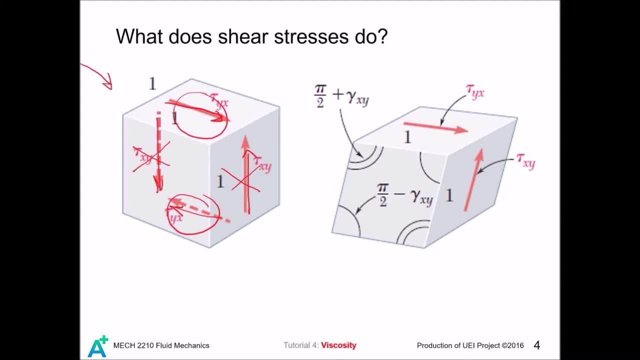 Then this pair of forces will generate a clockwise moment. So we need all four of them. After applying the four forces, we find that the cubic element element is no longer cubic and there is some angular deformations here. this angle is called shear strain. now we are back to our business. let's do an 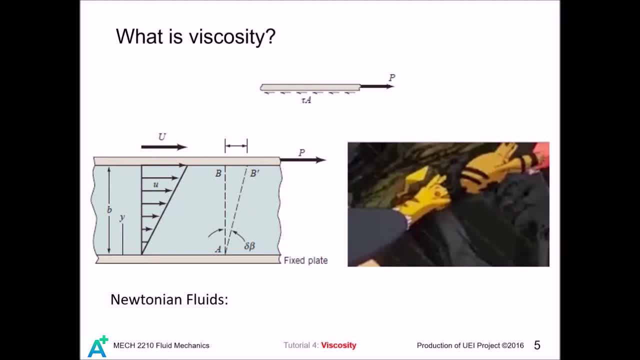 experiment. if we put some fluid between two fixed parallel plate and pull the upper plate with a force P, then a linear velocity profile UY is resulted. note that the particle at the flex plate is not moving. it is going to stick to the plate. this is called the no slip condition and you are going to use it in. 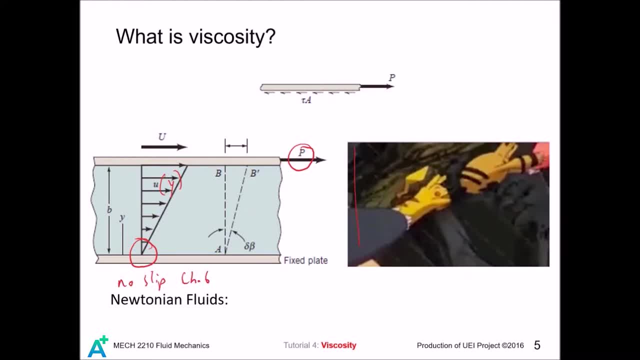 chapter 6 to make sense of this linear velocity profile. we can imagine that the particles do not want to be blown away by the current, so the proton particle will stick to the plate and drag the particle above it to prevent it from moving. so the velocity decrease as we go down. 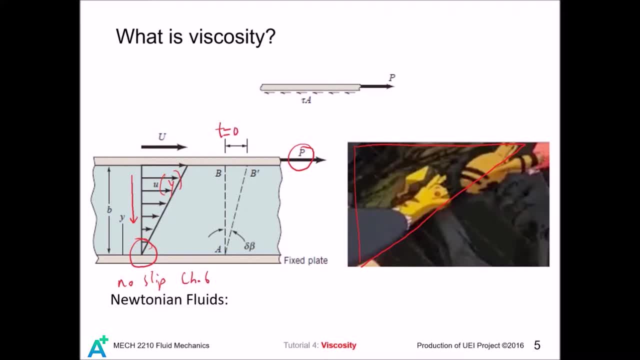 say, this photo is taken at t equals 0 and we mark down the position of the particle along line AB and this guy is here and after some period of time, t equals delta t. this particle will move here and this particle will move here and this particle will just stay here. if we imagine that we have a block, 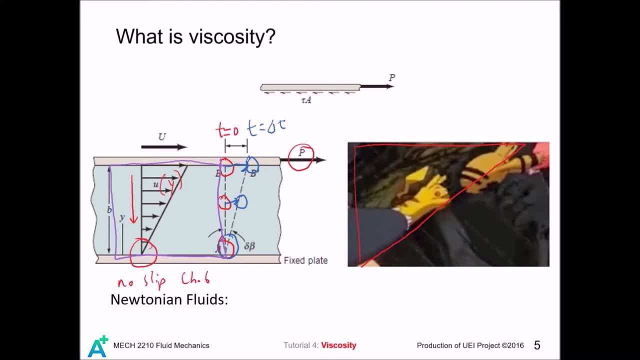 of fluid particles. after this period of delta t, our block of fluid particle will become like this: our block of particles has deformed angularly and this angle- we shall denote it as delta gamma- is the angular deformation of this block of particle. so what is this angular deformation? we have tangent delta gamma equals this length. 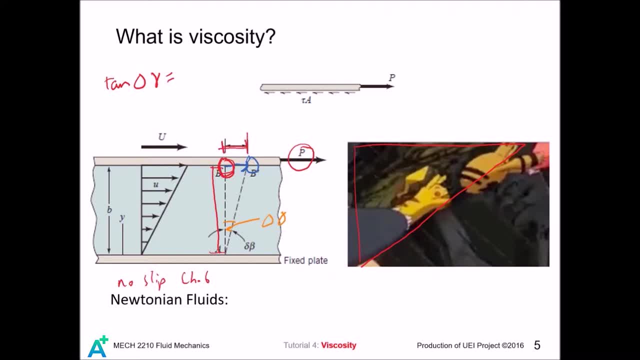 divided by this length, and this length is how much this guy has moved after delta t. so this distance is u delta t and this distance is b, and we have tangent delta. gamma equals u delta t divided by b. we imagine that delta t is a small period. 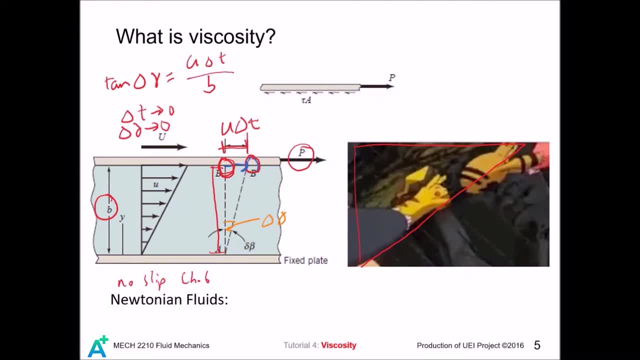 of time and this will also go to 0 and this tangent will just go away. and if we flow the delta t to the left hand side and take limit, this becomes gamma dot and is equal to u over b. but note that u over b is the slope here. 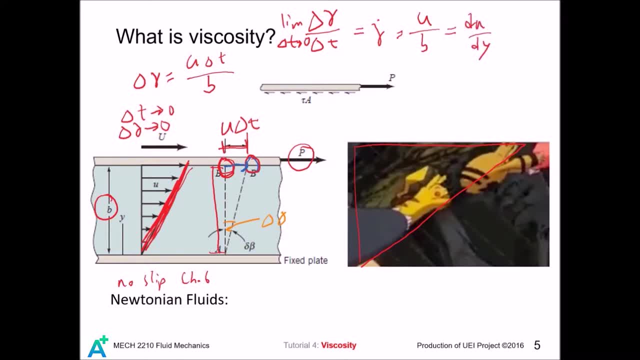 so this equals du dy. note that fluid, by definition, continually deforms, so it only makes sense to talk about the shear strain rate and that is gamma dot. we don't talk about this particular angle here, but in fact we know how much force we have applied and the force we applied is balanced by the shear stress on the plate. 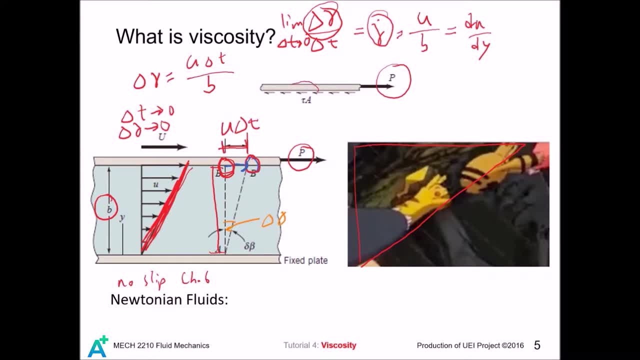 and the force we applied is balanced by the shear force contributed by the shear stress on the plate, where a here is the area of the plate, and if we continue our experiment, we find that for newtonian fluids, tau equals p divided by a, and that is proportional to. 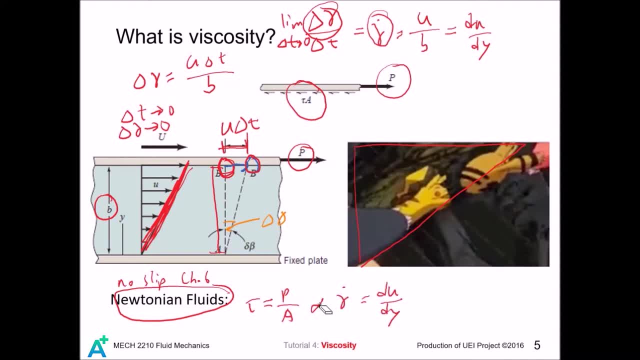 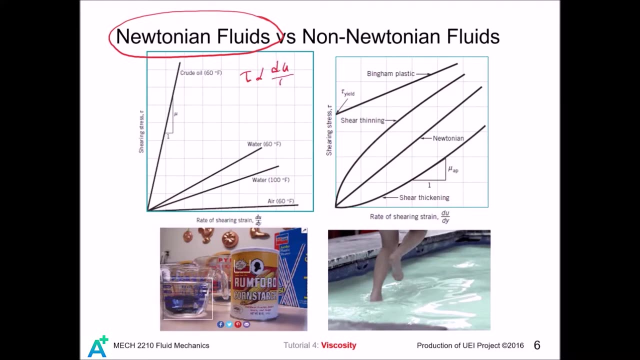 gamma dot equals du dy, and scientists left the proportionality constant as mu. that is the viscosity. so for newtonian fluid we have tau, equals mu, du dy. for newtonian fluids, shear stress is proportional to the velocity gradient, since these guys are newtonian fluids. 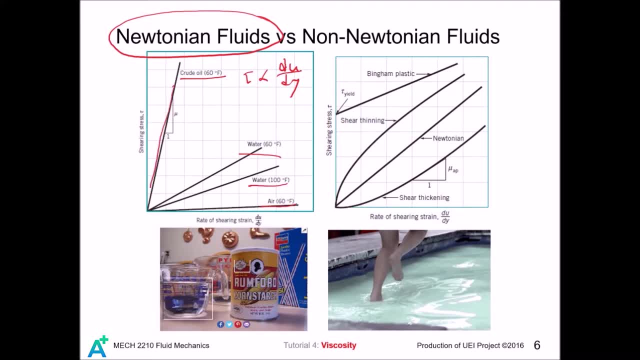 the tau du dy plot are straight lines and the slopes are viscosity. but in the world there are non-newtonian fluids, and corn starch is one of those shear thickening fluids. who can even work on it? but in this course we are just dealing with newtonian fluids. 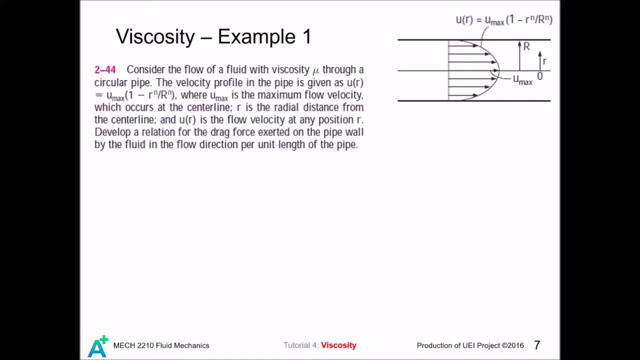 so we now do our first example. the question asks for drag force on a pipe wall. so we have to find the shear stress at the pipe wall first. in our symbol that is tau r, and we have just shown that tau equals mu du dy. but since we are using cylindrical coordinates, it is: 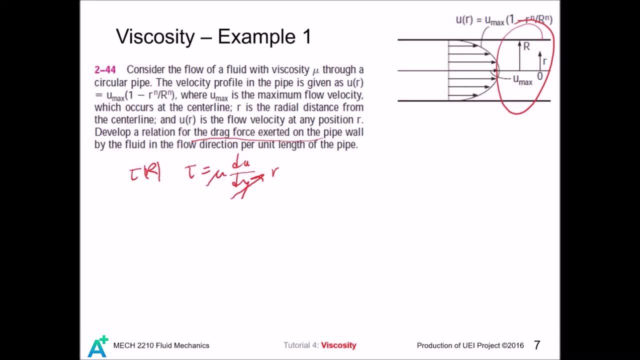 natural for us to replace y by r and let us just take the derivative of u u prime: r equals u max. one goes to zero and we apply the power law. since we are just interested in the magnitude, we take absolute sign and drop the negative tau. r equals mu du dr and r equals r equals mu u max. and divided by r and we multiply, 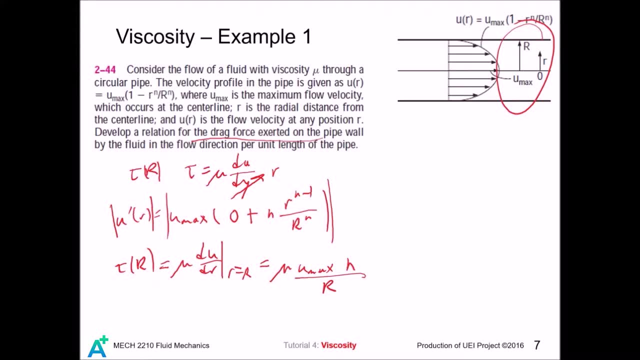 the shear stress by the internal area of the pipe. so we have: force equals two pi r l times tau. r equals two pi r l times tau r equals two pi r l times tau r equals two pi l, since the r cancels out times mu u max n and the question asks for force per length. 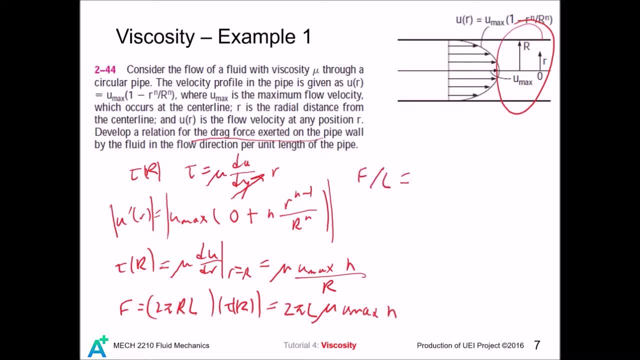 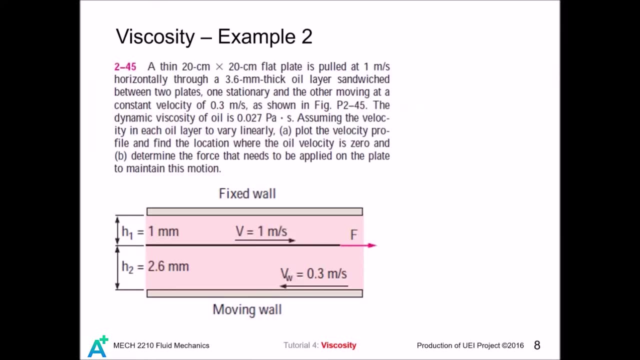 so f divided by l equals two pi, mu, u max times n. and that is our final answer. and let's look at a second example. the question requires to sketch the velocity profile and location where the oil velocity is zero. and if we do a rough sketch it's going to look. 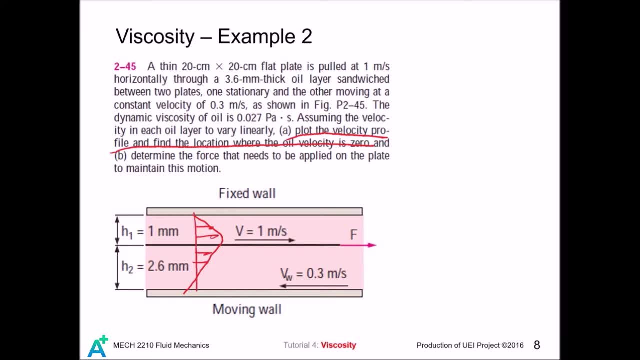 like this, since the profile is linear, and let's set our coordinate system like this and draw a more detailed sketch of u against y in the beginning is 0.3, go up and go down, and this is 1, 2.6, 3.6 and the units, and clearly we have a point of zero velocity to locate this. 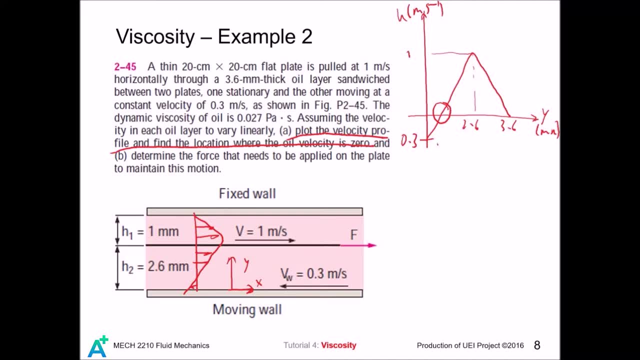 point we have to use high school math, so let's let this point point as 1, this point as 2 and this point as 3. we have go in the values and do some simplification and we found y3 equals 0.6 millimeters. 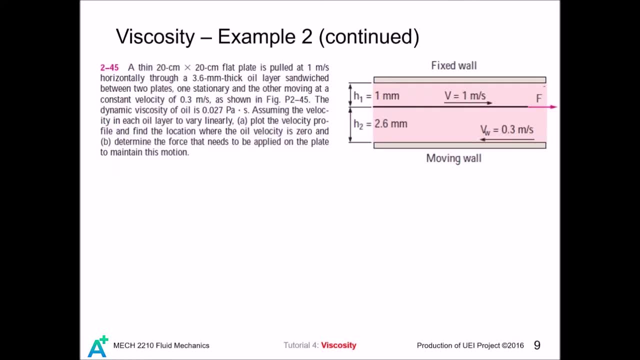 about the force. this time it's a bit different, since we are shearing stress above the plate and shearing will happen in different places, cause we are pressing the out of the, releasing the force, the gas stress below the plate, And we go on and calculate the shear stress above the plate. 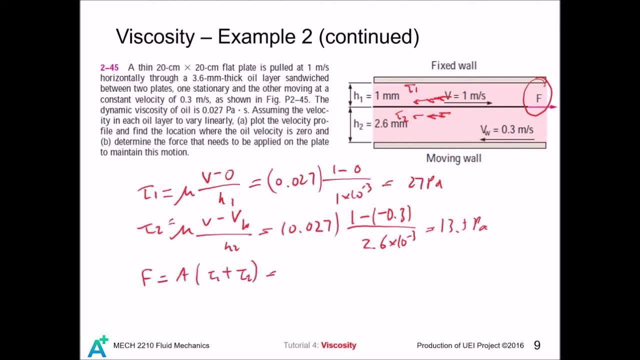 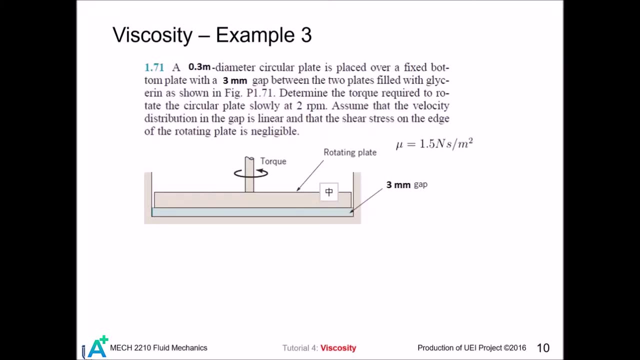 So that the total force is. And we are done with this example. Let's go on to do a final hard example. Hope this is not going to be on your exam. So let's look at this setup. Is there any plate moving at constant? 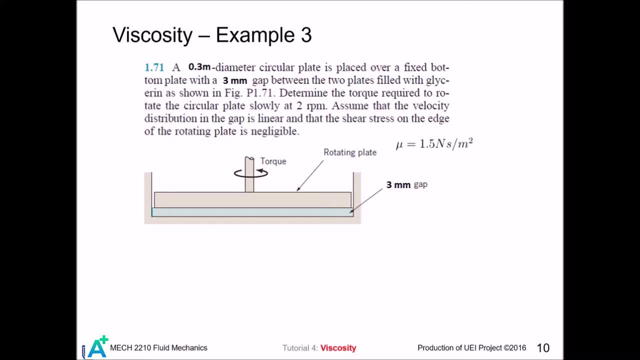 speed above a fixed plate with a layer of fluid in between. I will say yes and no. Yes, there is a fixed plate here and there is some fluid here, But certainly the rotating disk here does not have uniform linear velocity If we draw the upper disk. 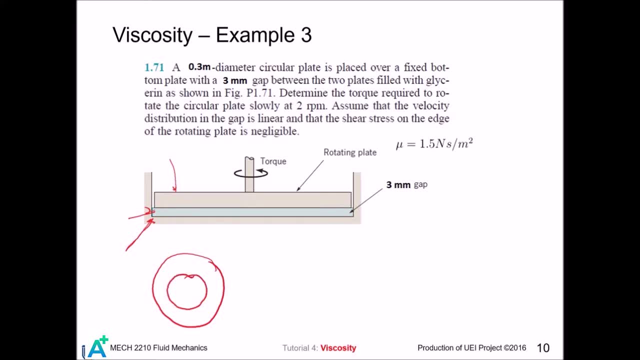 in a small circle here for reference, and we denote the radius of this small circle as R, And we pick two points here, 1 and 2, then velocity of point 1 is R omega. V2 equals R omega, So the rim is moving faster than the interior. Let's also draw the 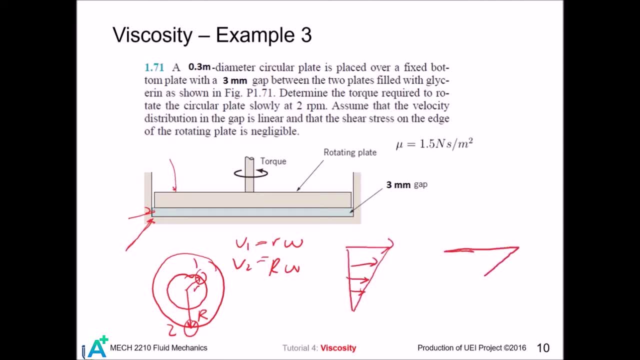 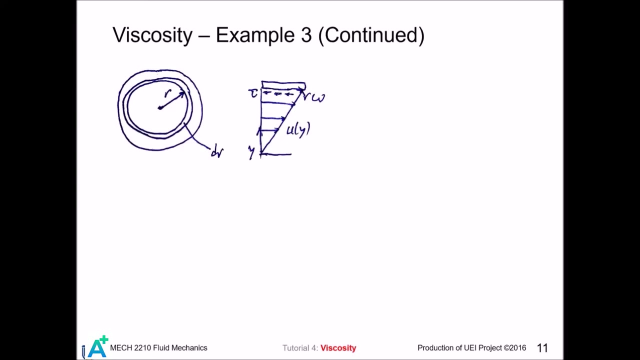 velocity profile of the fluid under the under points 1 and 2.. And this is V1, this is 1 and 2. we can imagine that the point V2 is subjected to a higher shear stress than point 1, so we shall cut our rotating disc into rings of. 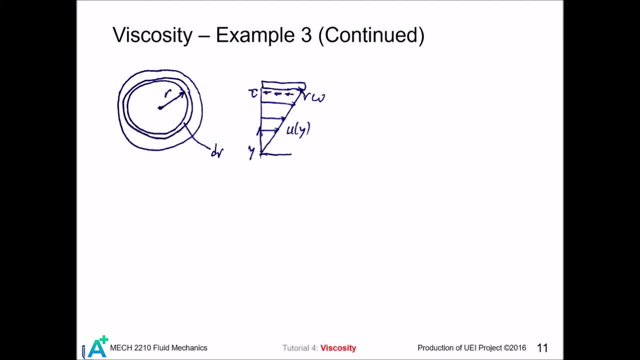 thickness, dr as shown, such that each is moving at uniform speed and we can calculate the torque dt on each ring, since torque equals to radius times force, and we can write: dt equals rdf and the drag force equals tau times area of the ring. so equals tau da and da is the area of the ring, so it's 2 pi r times dr and we 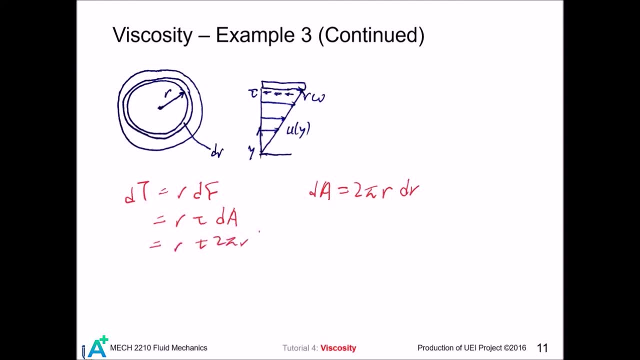 can put it in and becomes 2 pi r dr. and tau equals mu times the velocity gradient and that is mu times r omega divided by B. and we plug it in and this whole thing becomes 2 pi mu omega B r cubed dr. then we combine this: 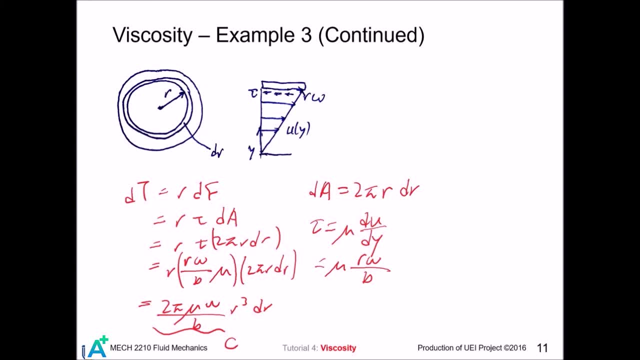 constant as C, then we can integrate. for the overall torque, we integrate 0 to r dt and that is now you can see that the modulus is 0. and if i put angle here we can throw Leaving Circles. here we don't have to, we can put this solution. okay, we got extrovert. 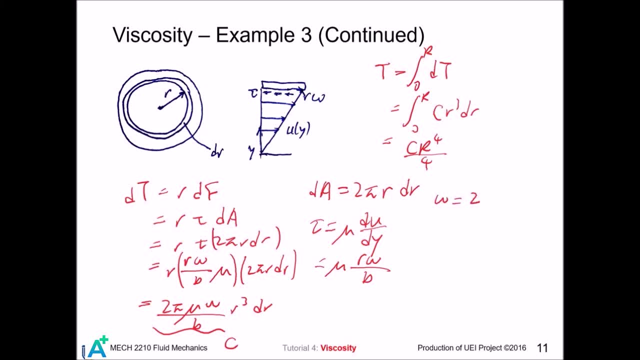 ahonielevert ½ belt, just the decrease, the starting line, which we found to be earlier, and we can also do it fornik seasons can add the two, the V2 components, fromhand line of the ring frequency to the logarithmic interval, so we can. 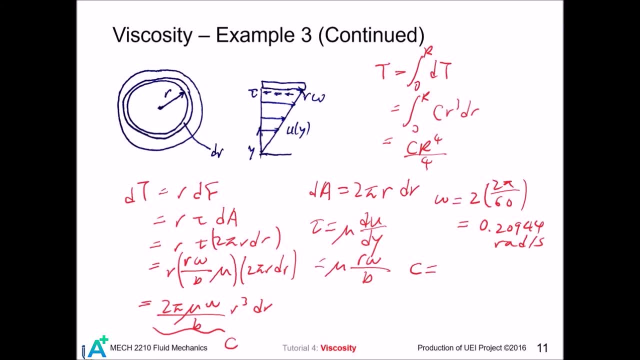 calculate 1 by 2 pi: 1: 1. so we have 1 by 2 pi and another constant fornik time. on the right hand side we do have 1 by 2 pi. very well, but i forgot to talk about the Jub valtrick formula, because it gives the relative one, that is, 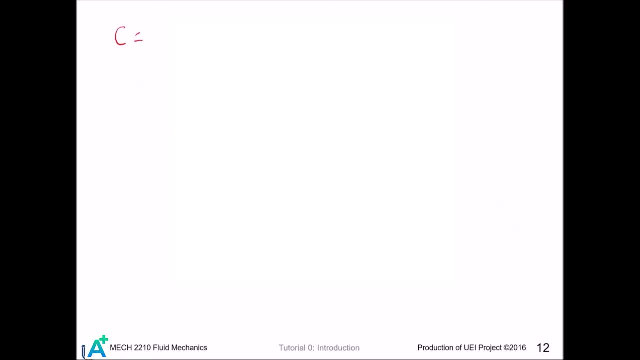 equidistant and we don't need the свою formula, we only need r cross theta, we go So, basically. So we melting the center, we have a constant r, 2 pi and we name isトу π. Punching the calculator, we find that C equals 6,, 5,, 7, or 9,, 8 newtons per meter cube. 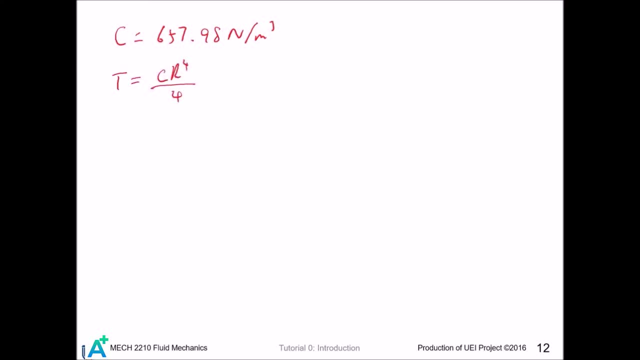 And we find that T equals Cr4 divided by 4,, and that is radius, not diameter, divided by 4,, and that is 0.0833.. So today we covered an important free property called viscosity. We did a review of shear stress and strain in order to discuss the definition of viscosity.